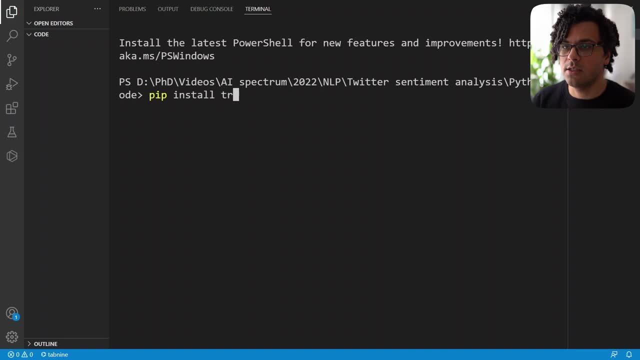 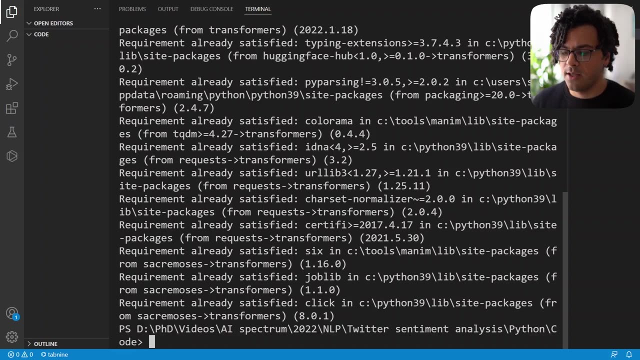 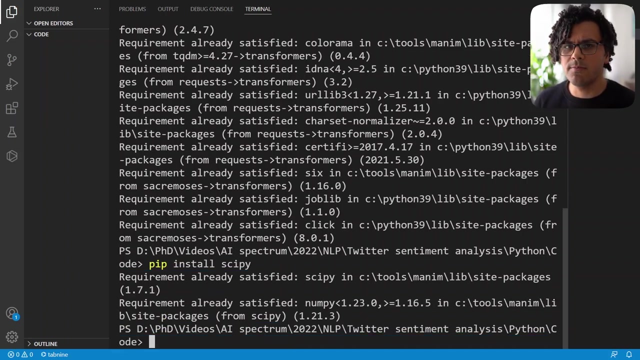 over here. first I write peep install transformers. We use this package to download the model from the Hugging Face website. and then I write peep install scipy that we're going to use it to convert the output of the model into probability scores. Now we have the packages, I create a new Python file. 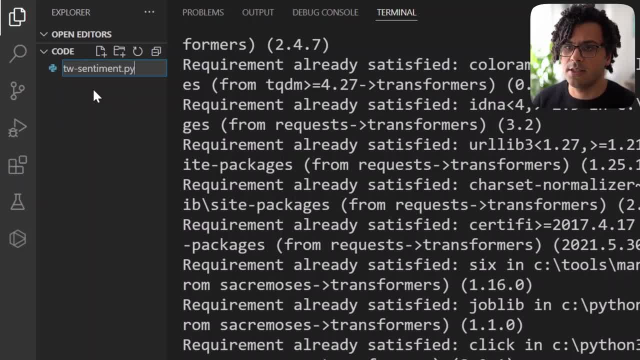 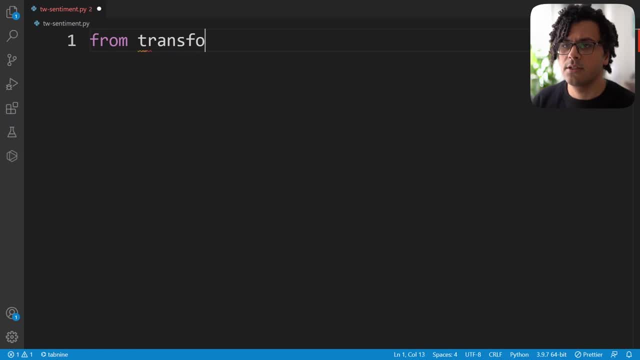 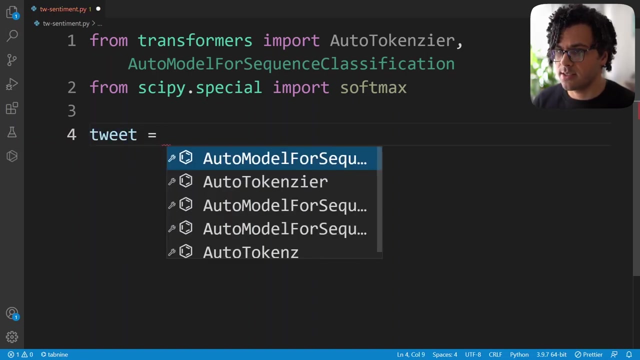 call it Twitter sentimentpy so we can start writing our codes. So I write from transformers: import auto tokenizer, also auto model for sequence classification. Then I write from scipy dot special import softmax. So now let's consider a tweet for our sentiment analysis. Now, when we are talking about the text data of a tweet, 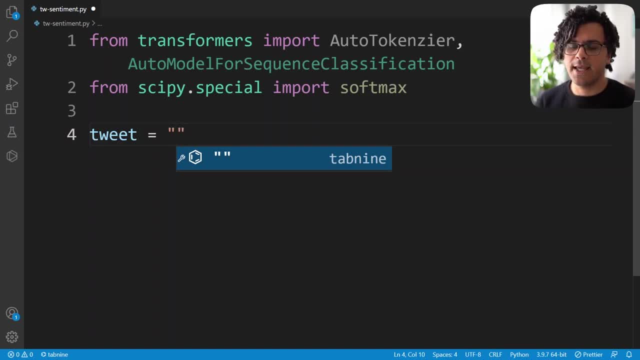 we can consider it into four categories. One is the text regarding the tweet itself, Then there is emoji, Then there is normally mentions of a user and there could be also some link to some website inside a tweet. So I write a tweet that has all of these components. So first, 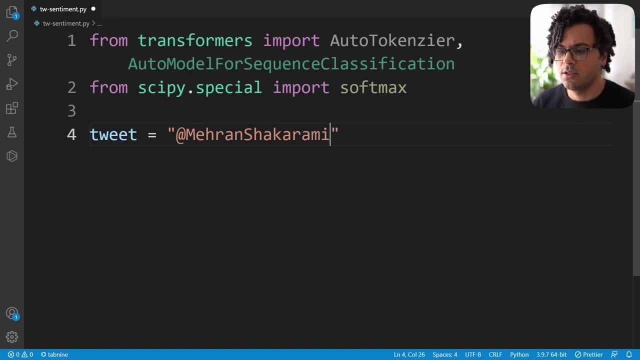 let's write a mention and then the tweet- for example, today's cold at home- and then I write also an emoji, For example a sad emoji, And then some link, For example the link to my website. So now we have the tweet and we'll use the Roberta model to see what's the 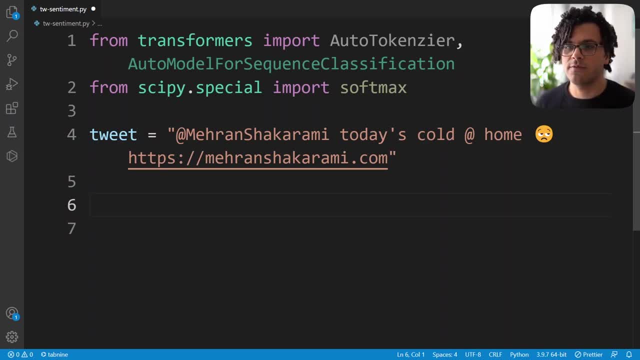 emotion of this tweet. Now, in order to do the analysis we should come, we should do some pre-processing on the text to make it appropriate for the way the model is trained. So the way this model is trained is, instead of mention of anybody, they just use at sign user. 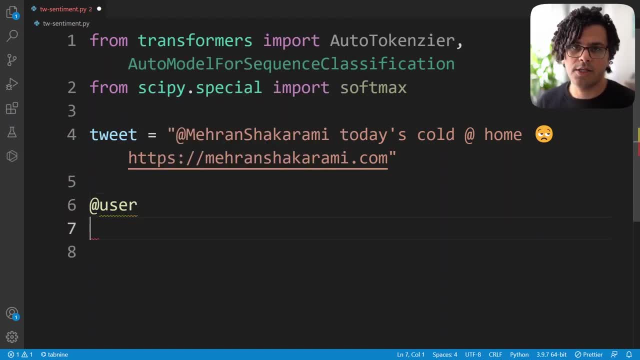 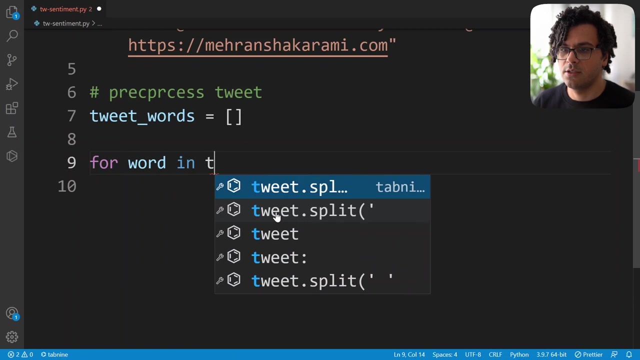 And instead of any hyperlink, which is any URL to any website, we should just write HTTP. So that's what we're supposed to do. So I write pre-processed tweet, Then I write tweet underline words as an empty list For word in tweetsplit, And then we split the. 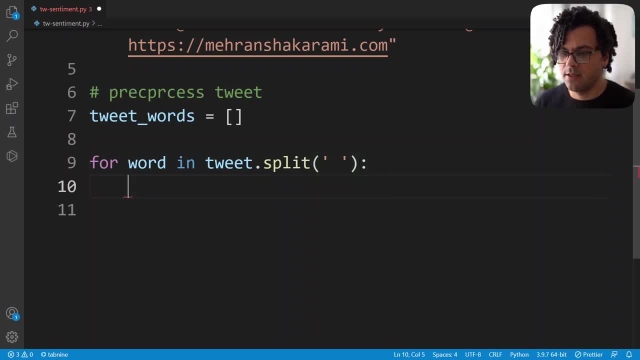 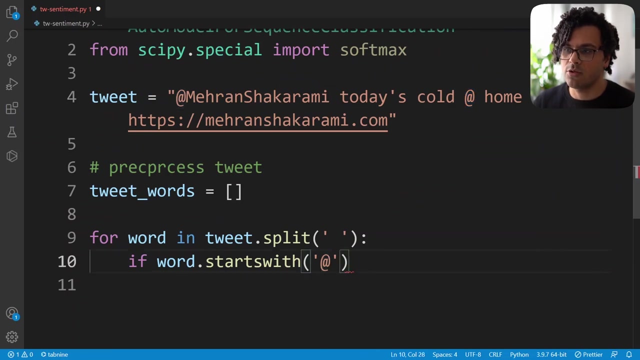 tweet text based on spaces. Then I say: if word starts with at sign, So that means it's a mention to somebody. But we see, for example over here we just have some at sign. that is not a mention, So we should also somehow exclude this one. So we see, if the word starts with tweet and its length. 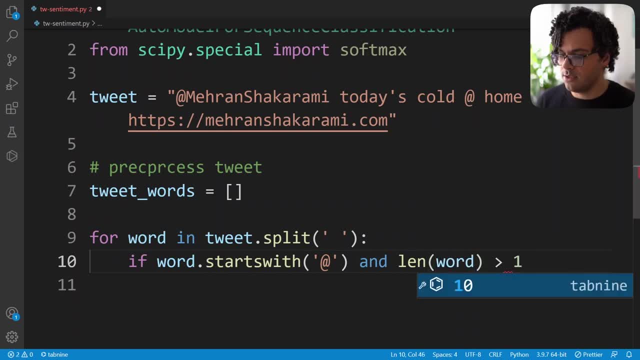 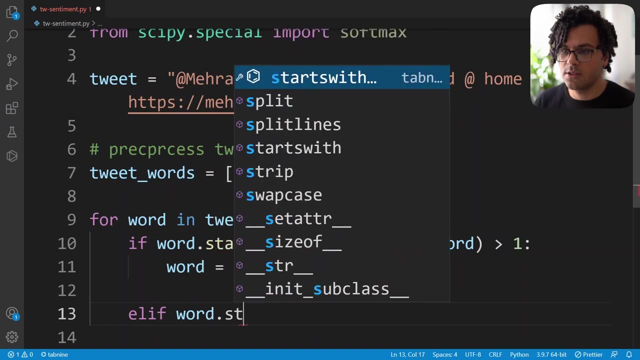 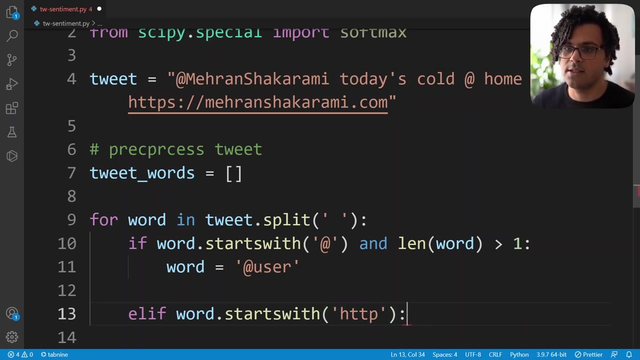 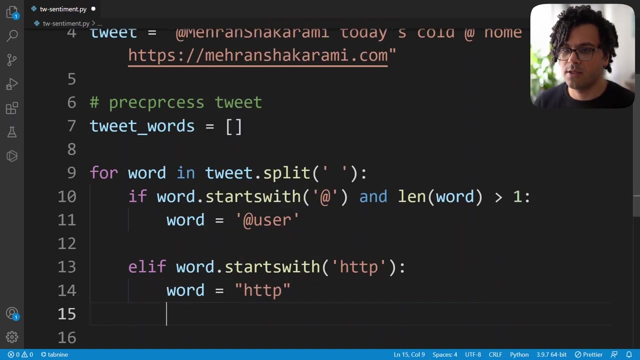 is greater than one, And then we convert it to a string at user. Then, similarly, we say else if word starts with this, time HTTP. So now, this time we are selecting the URL link, We convert it into a string, which is HTTP. Then what we're supposed? 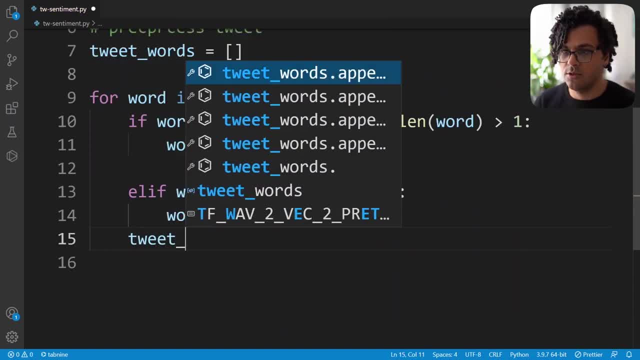 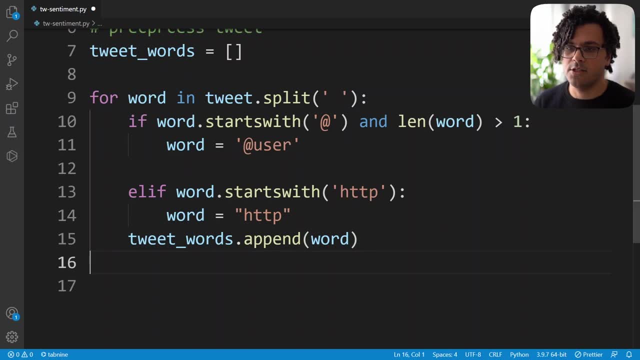 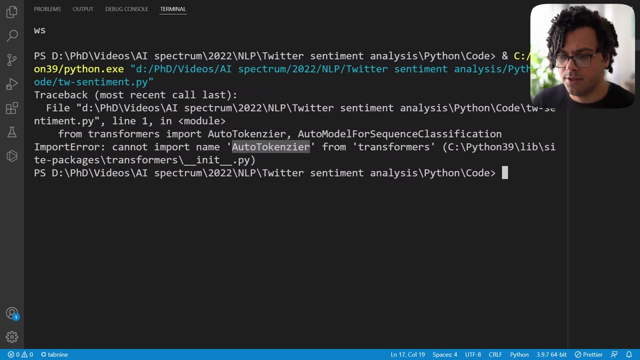 to do? we are supposed to add this to our tweet words list, So we append it to our tweet words list. Now, if I just print tweet words, We see it's a list that has all the elements over there. Oh, so I got some error. I think I have some sort of type over here: Auto tokenizer. Okay, 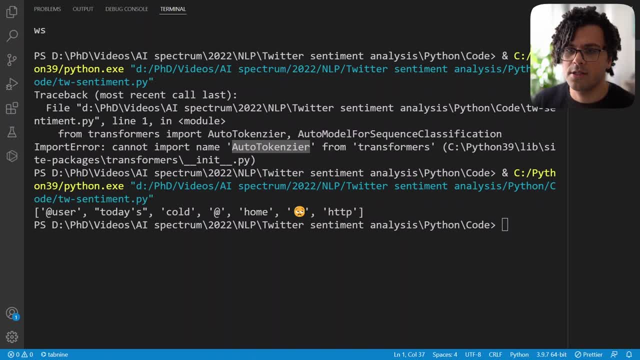 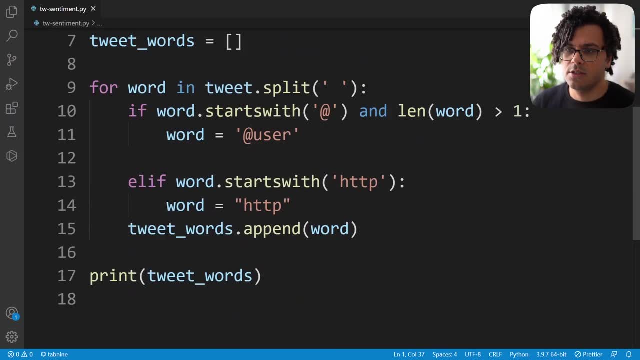 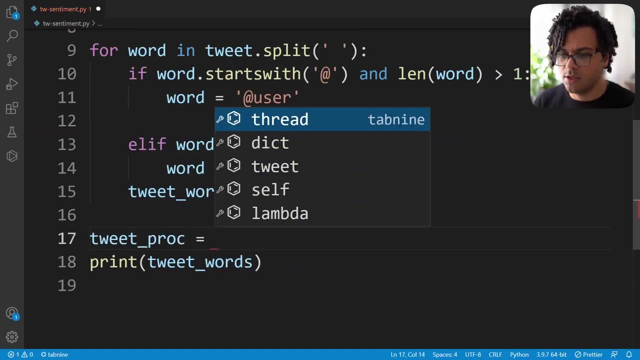 Now again, I run the code. OK, this time it works. Now we see we have a list of the tweets. Now we should just join all of these elements together, So we can do it by writing tweet processed equal to space string and then join our tweet words list. Now, if I just 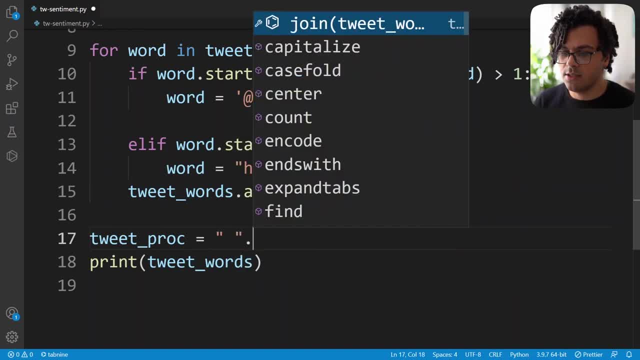 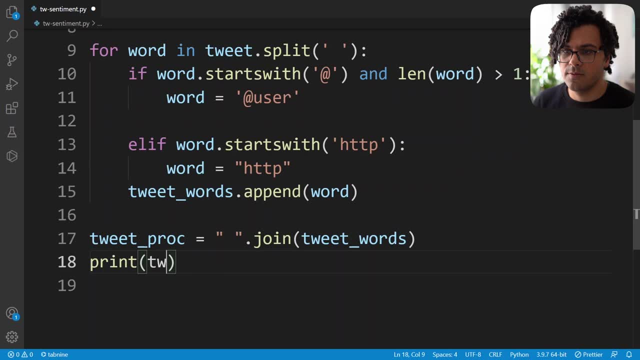 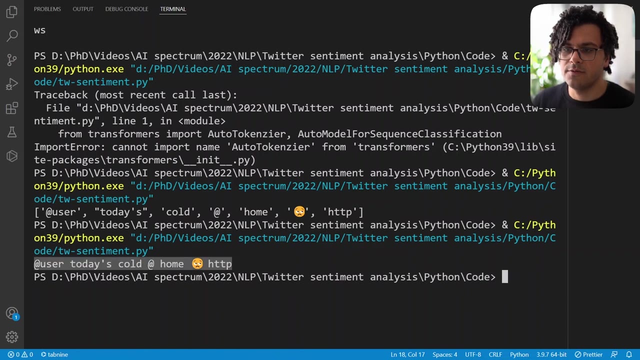 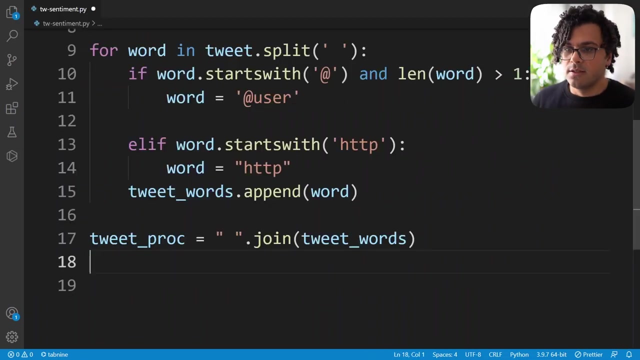 print this. So I am going to create third time neg method that says this: are actually now if I just print this one. yes, so now the text is converted. we got rid of the mention and also the link. now the next step. we should download the model, so we. 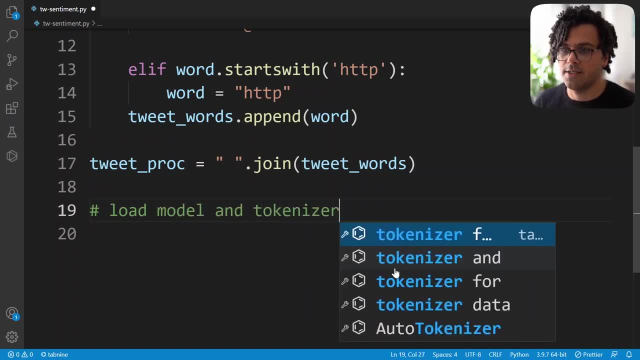 load the model and tokenizer. so now I write the name of the model- Roberta, I call it- and then I go to the hugging face website. I copy from here the name of the model so I paste it here. then I can now download the model from the. 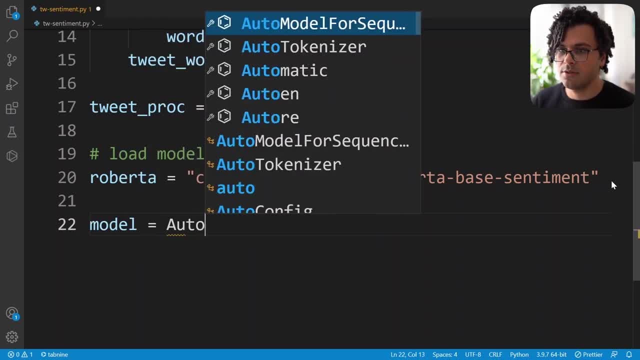 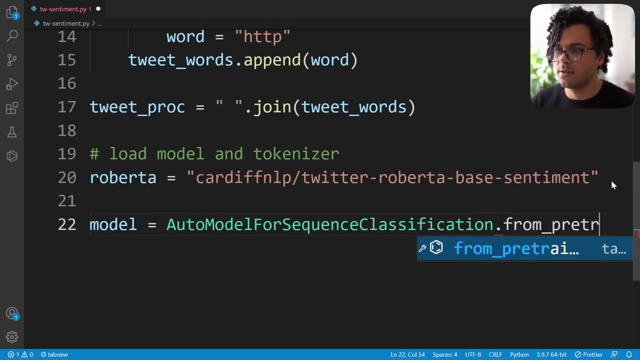 website. so I write model. then I use auto model for sequence classification dot from pre-trained and pass over here the name of the model. Roberta, we should also load a tokenizer so we can convert our tweet text into appropriate numbers. so we can then pass the numbers into the model. so I write tokenizer. 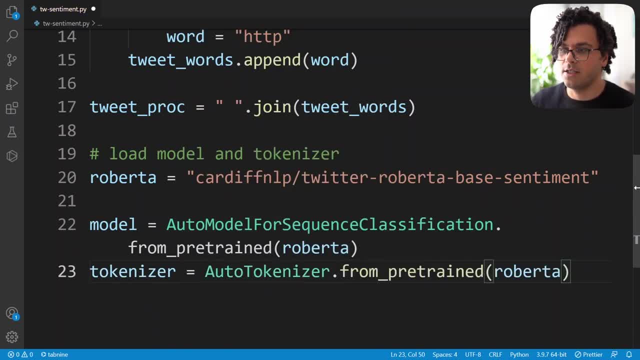 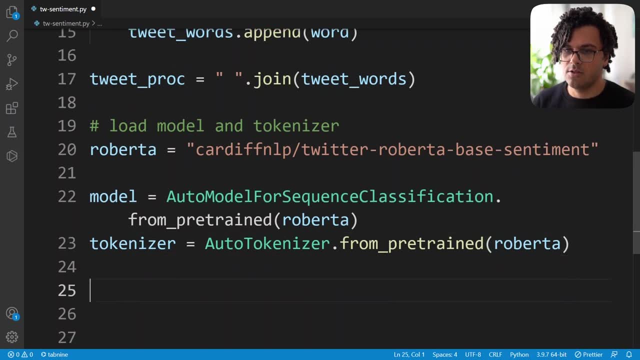 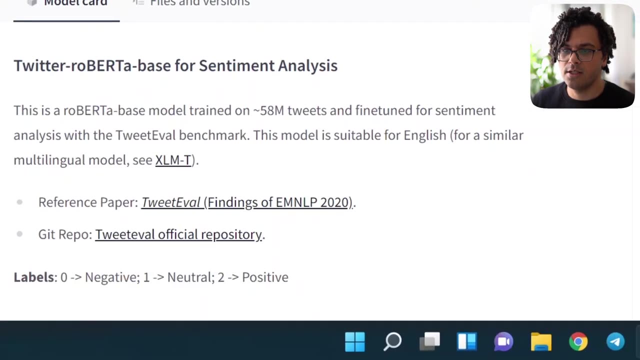 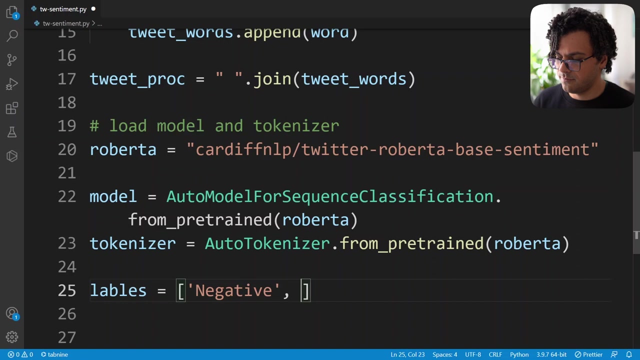 auto tokenizer from pre-trained and again pass over here the name of the model. now I also write the labels of the output of this model. so I make a list called labels and then from the website we see the labels are negative, neutral and positive. write them here: negative, neutral and positive. so now we can write our code. 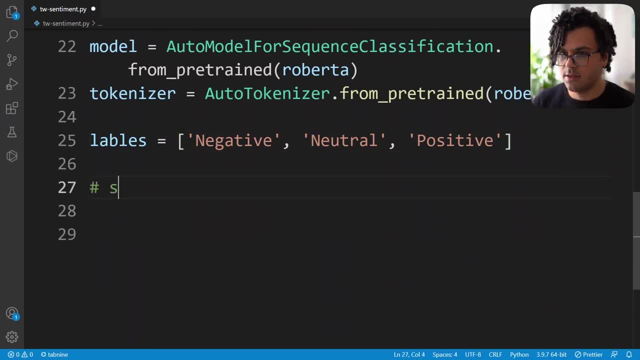 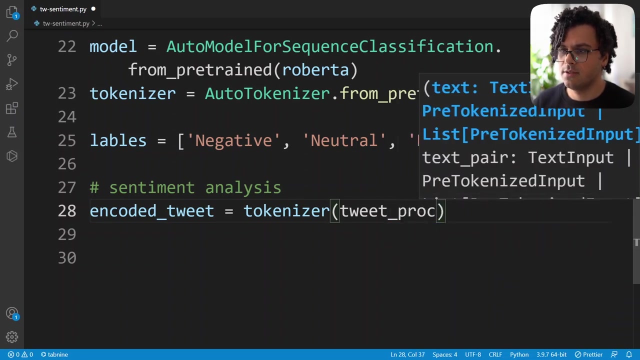 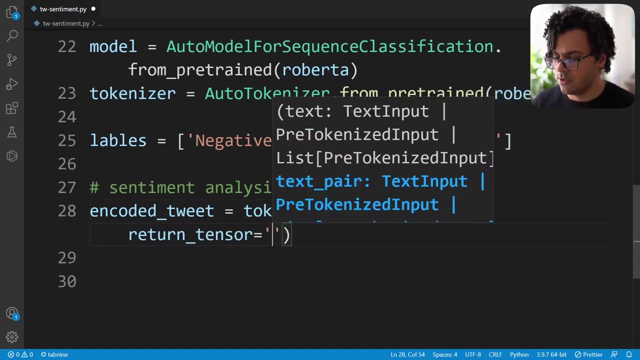 for tweet sentiment analysis. first I convert this process to it into pytorch tensors and then we can pass that into the model. so I write encoded tweet equal to tokenizer, pass over here the tweet processed and then return tensor is equal to pt. so let's just print this encoded tweet. 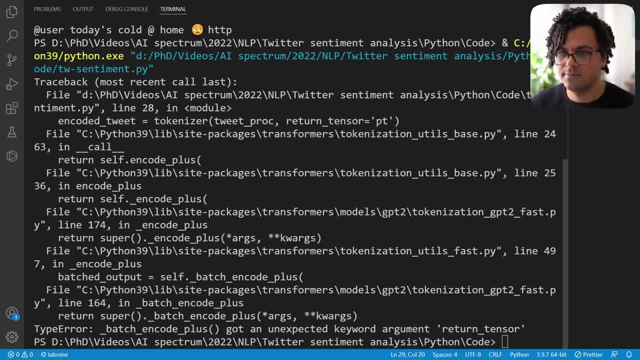 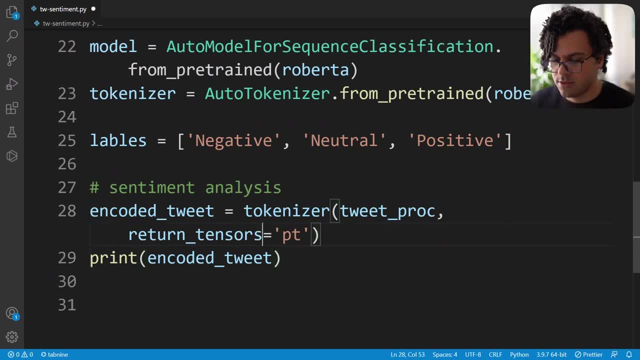 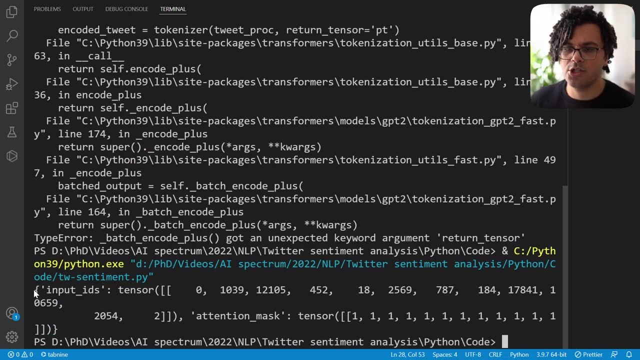 see what we get. so we got some error over here. it should be return tensors, not tensor. now again we run the code. so you see, the encoded tweet is actually a dictionary. we have input ids and attention mask and then the input ids is actually the tensor that is obtained from converting the tweet into. 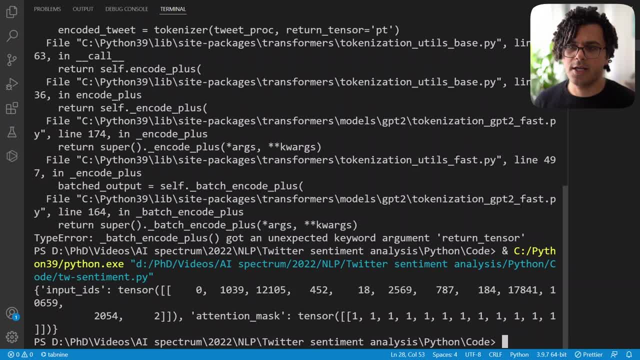 numbers. just have in mind that when you are running the code for the first time, it might take a bit longer because you need to download the model from the website, But then after that you wouldn't have the problem because you already have the model. So now we should just 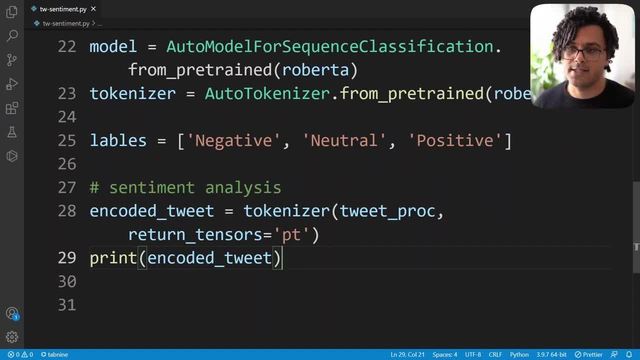 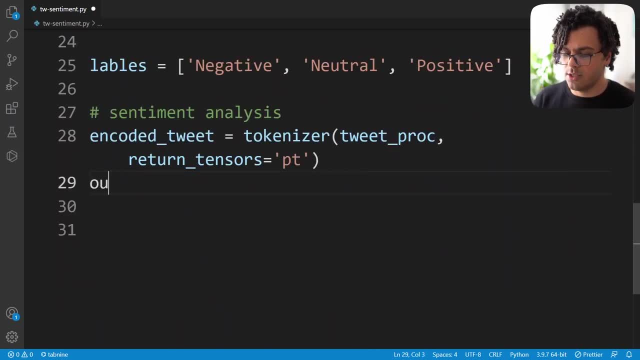 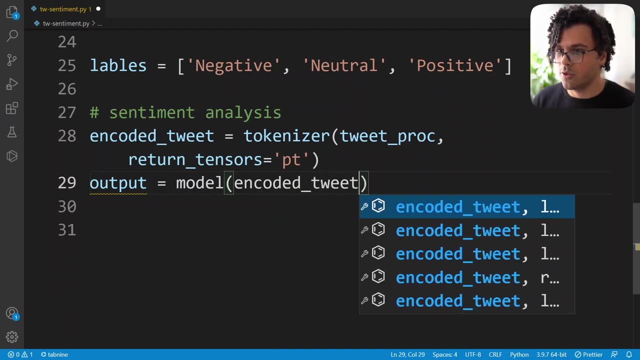 pass this encoded tweet to the model to do the sentiment analysis. Okay, so I remove this line. So one way to do this: I just write output model and then pass over here encoded tweet. Then I write the keys of this encoded tweet. So over here we have input IDs. 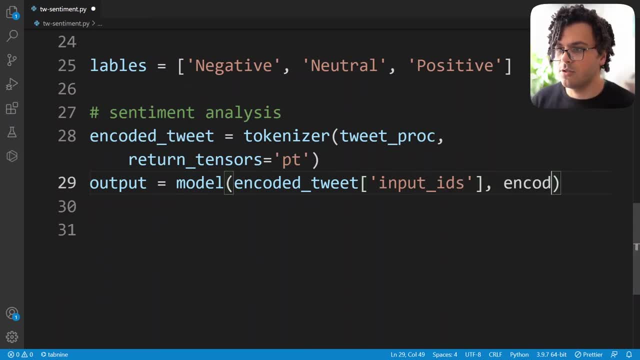 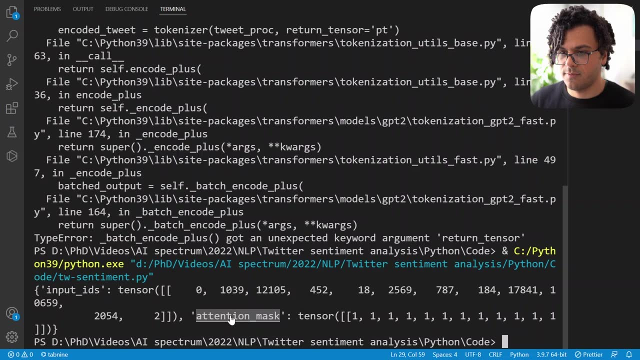 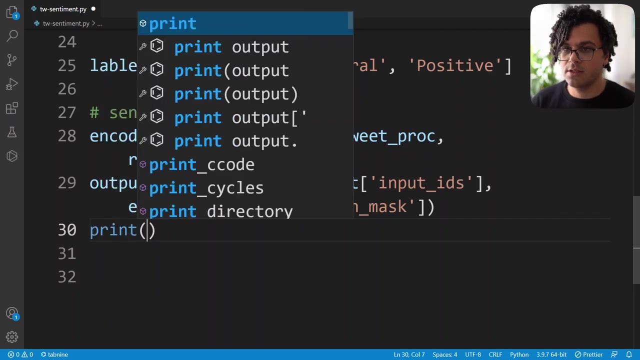 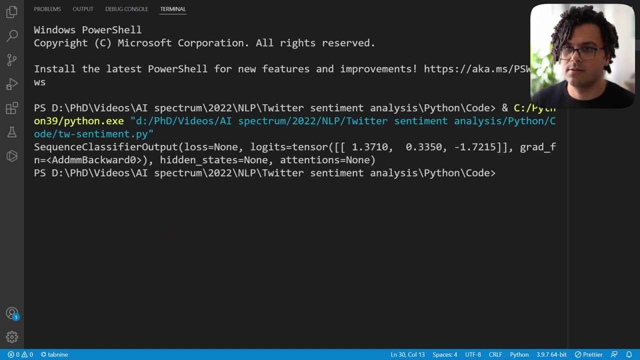 I put it over here And then again encoded tweet Again, pass over here attention mask, So that's a way of writing it. And then, if I just write print output, you see that it does this Sentiment analysis. So here is the output of our analysis. We have a tensor over here and we will convert this into: 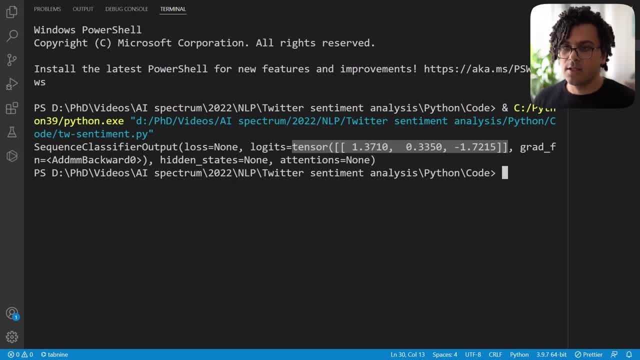 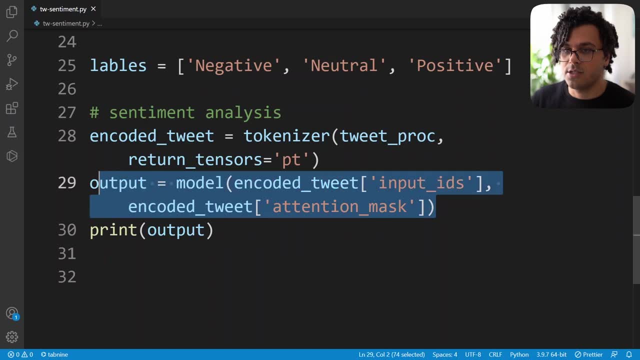 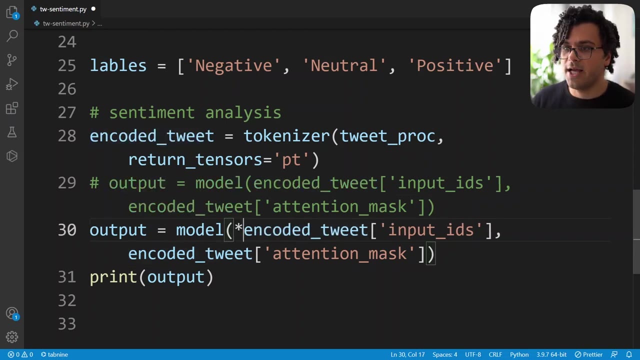 probability to see exactly what's the sentiment of the tweet. But instead of passing the encoded tweet to the model, we can actually do something much simpler. I can just copy this part And then I comment this. Instead, we can use this double asterisks, which is doing exactly the. 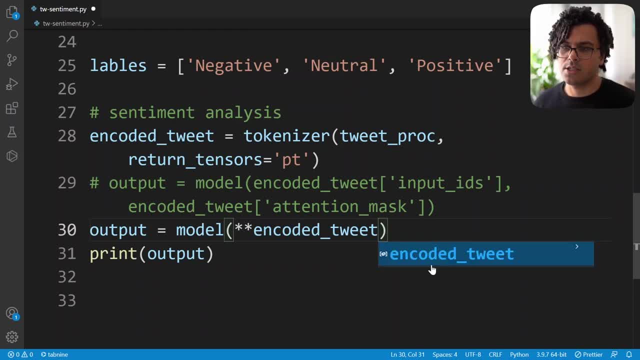 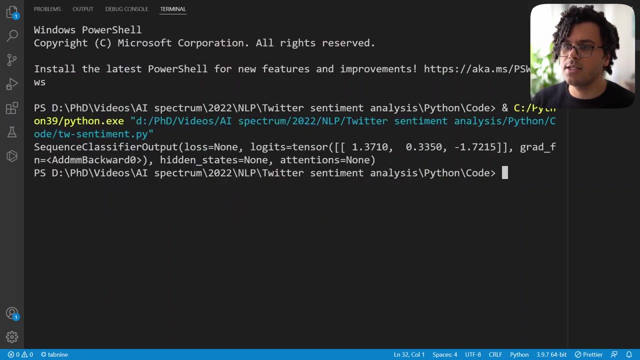 same thing that we do. So this way we unpack this encoded tweet dictionary and then pass it to the model. Now we have the output of the model. We can convert it into probabilities using softmax and see what's the sentiment of the tweet. So what I'll do first is to select this inner list over here. 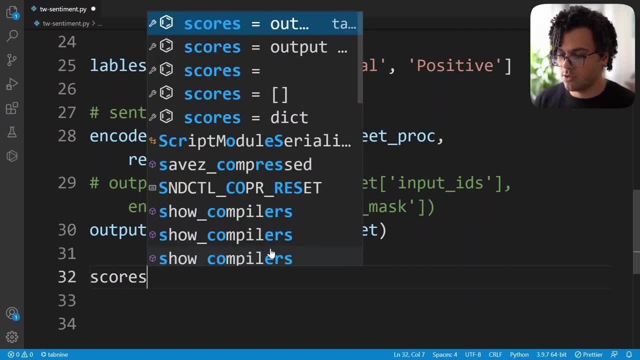 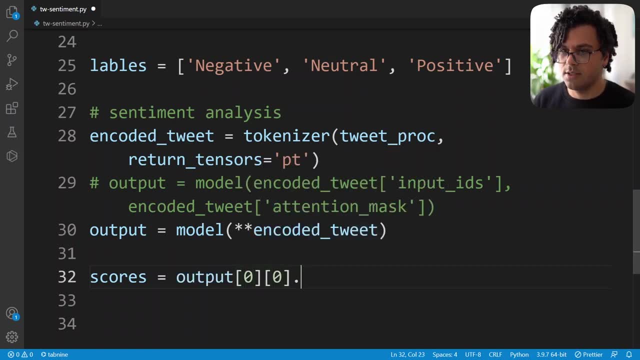 To do this I write scores equal to output zero, zero, And then I write detach to just select the list And then I just compare it into a NumPy array. Now, if we just print these scores, we see we have selected the list that we want. 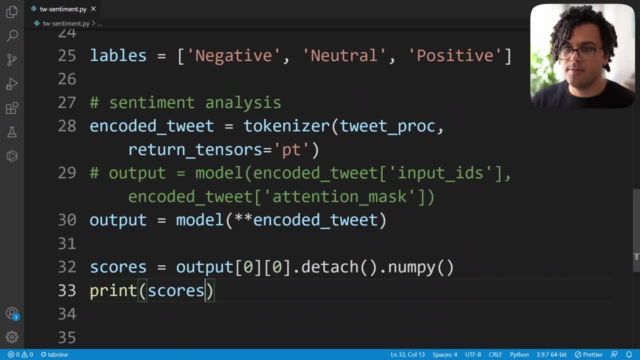 And here we got it. So now the next step. I will pass these scores into the softmax function. So I write softmax scores and convert it into probabilities. If we again pass it, we will get only numbers between 0 and 1.. 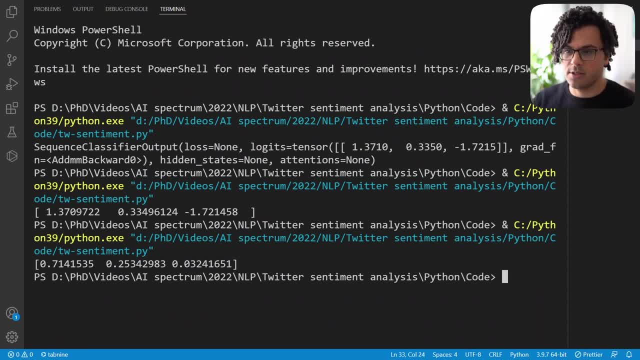 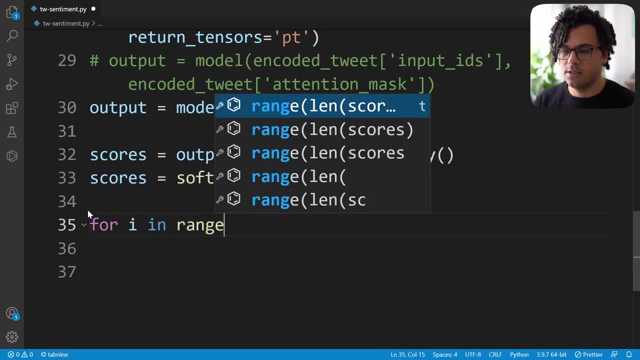 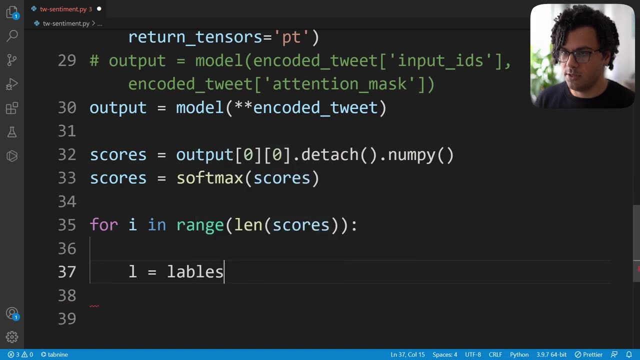 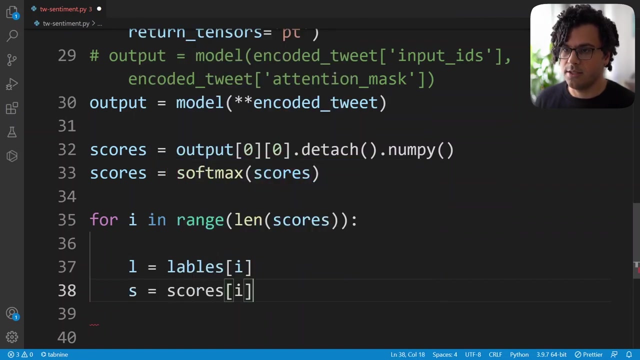 So now we just need to print the output with the corresponding labels. For this I just write 4i in the range of the length of scores, L equal to labels the ith element, And score by s is the scores ith element, And then I just print. 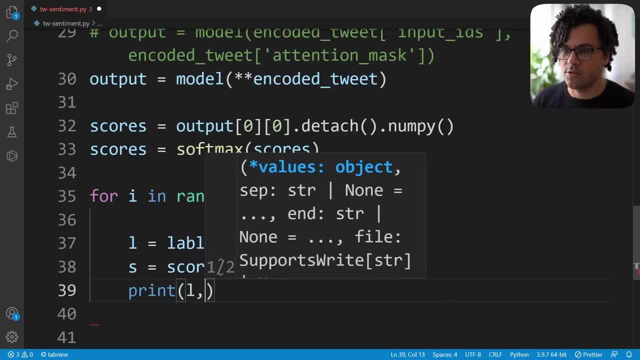 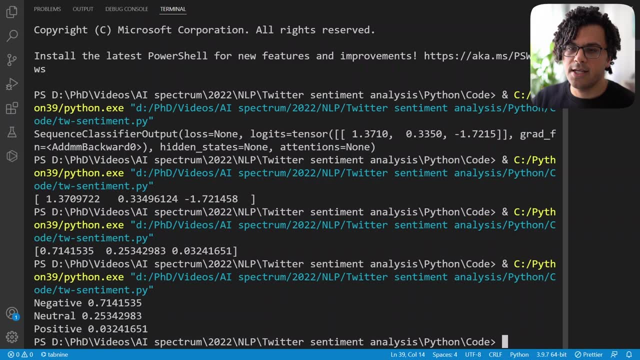 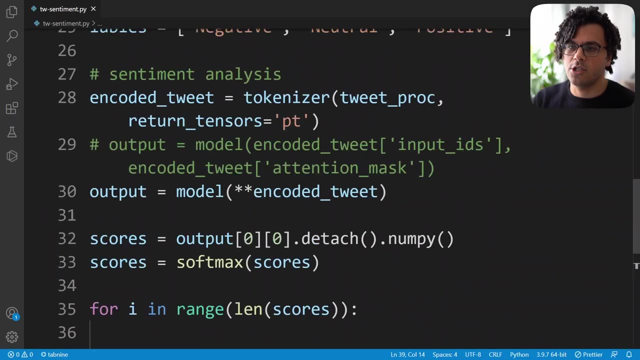 the label and the score. Now we run this code And we see the scores and the labels of the output. So we see that the label of this tweet is negative because it has the higher score, And that's again as expected If we go back to the python code and change the tweet, for example, to a positive tweet.